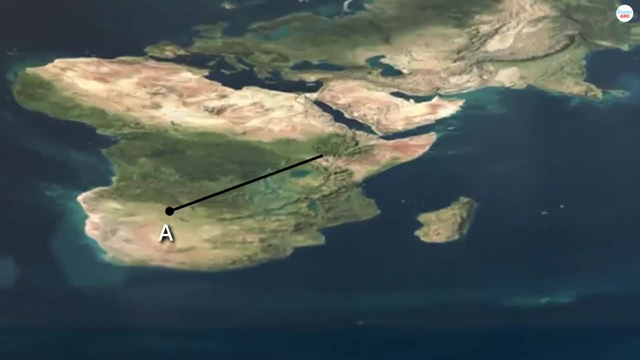 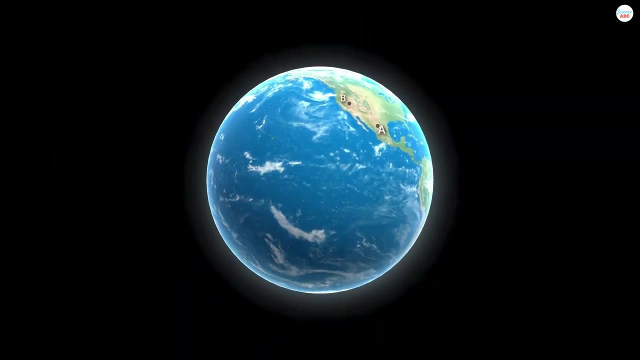 earth, which we don't, then yes, a straight line would be the shortest distance between points A and B. However, the earth is an approximate sphere and the shortest distance between two points on the surface of a sphere is an arc known as the Great Circle Distance. 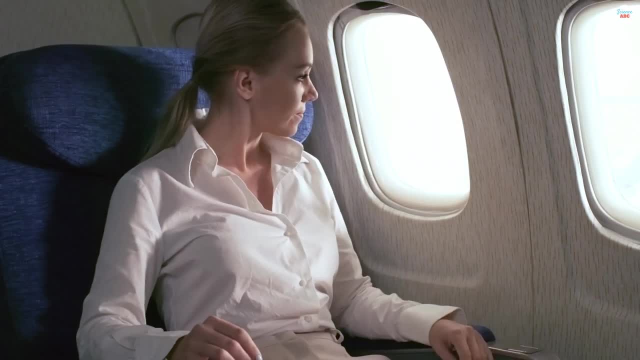 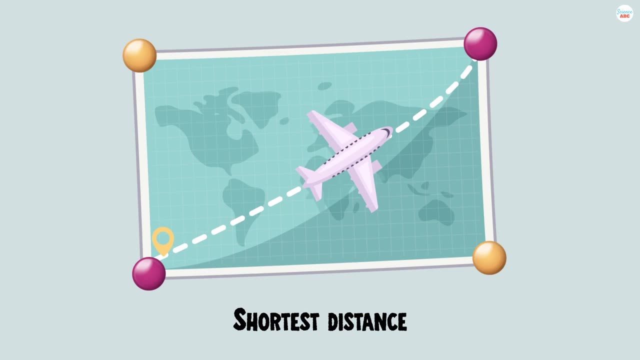 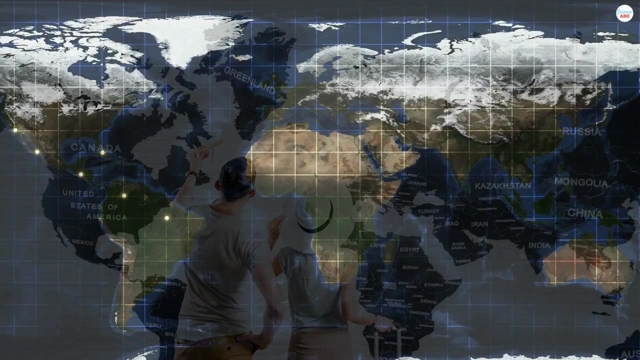 People who have traveled by air have likely noticed that flights don't follow a direct path, but instead take a curved route to their destination. The curved routes are used because they're actually the shortest distance between those two locations on our planet. These curved routes are often confusing, as the routes are outlined on a flat. 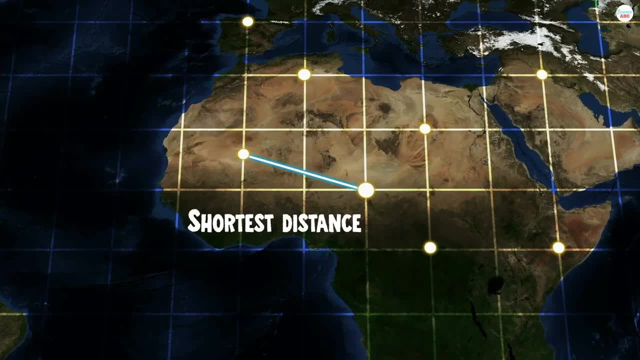 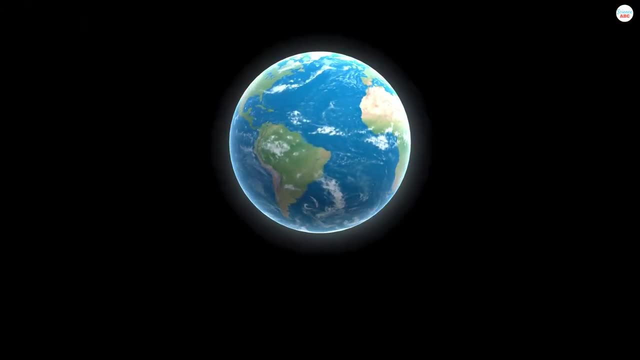 two-dimensional surface. The curved routes are often confusing, as the routes are outlined on a two-dimensional map where a straight line might appear to be the shortest distance. However, a two-dimensional map of the earth can never be entirely accurate. Earth is a three-dimensional space and is best represented using a model globe. 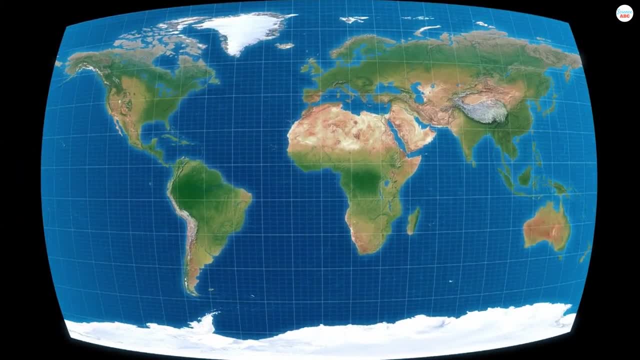 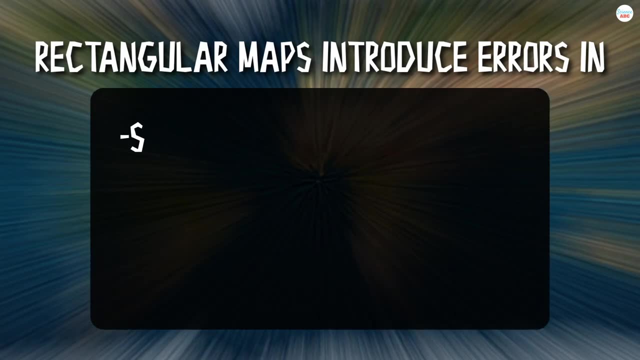 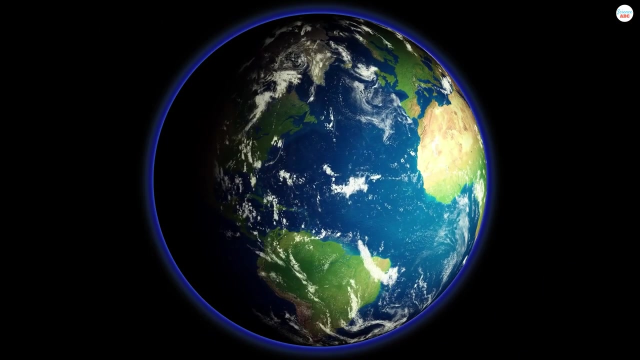 However, when one tries to flatten the sphere into a rectangular shape, as most maps do, the age-old dilemma of distortion arises. Most rectangular maps trade country shapes, sizes, intermediate distance and even legitimate information for ease of understanding. On a globe, the shortest distance between New York and Paris would be an arc of. 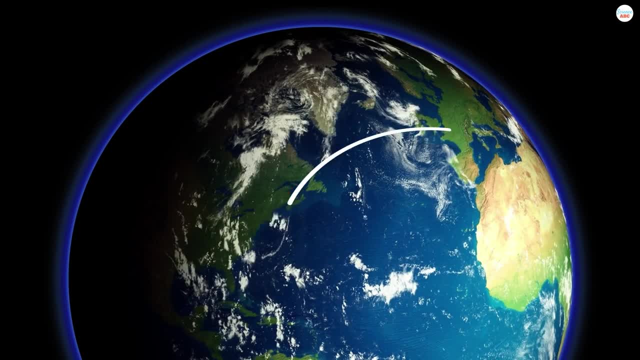 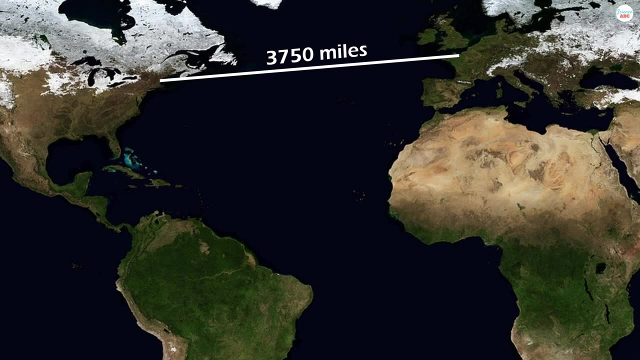 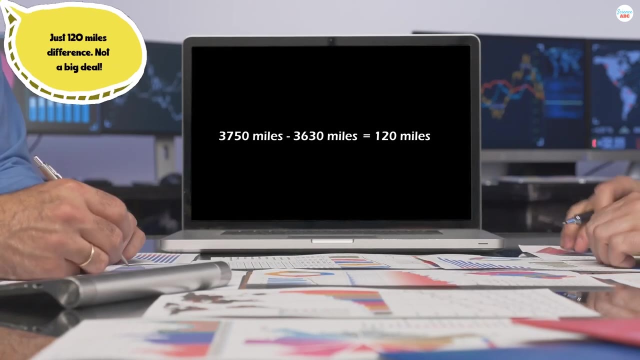 roughly 3,630 miles, But the same arc, when projected on a 2D map, transforms into a straight line measuring approximately 3,750 miles. The difference between the two numbers- roughly 120 miles- may not seem like a big deal, But considering the fact that a Boeing 747 consumes an average of 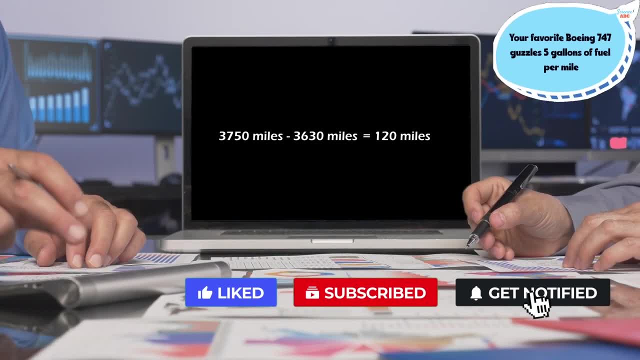 five gallons of fuel per mile in the air. the difference between the two numbers- roughly 120 miles- may not seem like a big deal, But considering the fact that a Boeing 747 consumes an average of five gallons of fuel per mile in the air, the difference between the two numbers roughly 120. 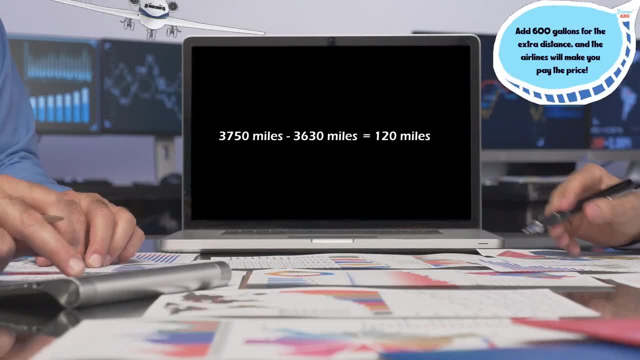 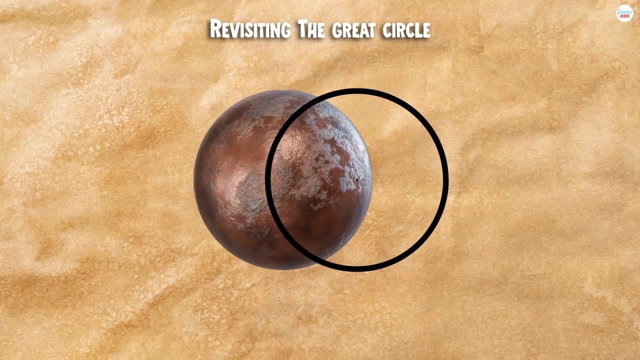 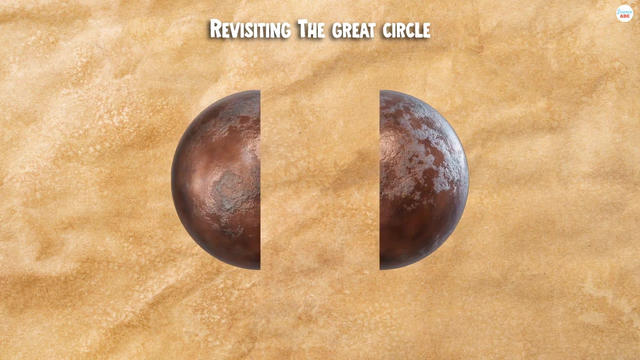 miles may not seem like a big deal, But considering the fact that a Boeing 747 consumes an average of- In purely mathematical terms, a great circle is any circle drawn on a sphere whose center coincides with the center of the sphere, thus dividing the sphere into two equal halves In simpler terms. 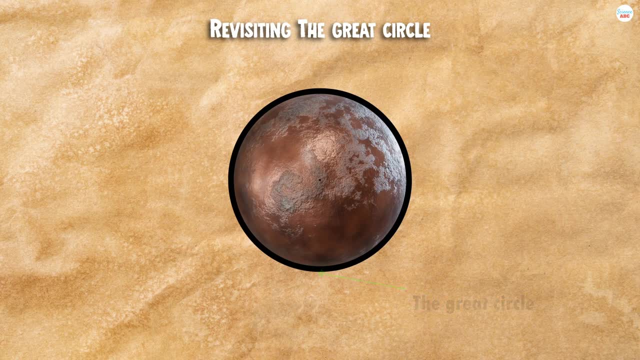 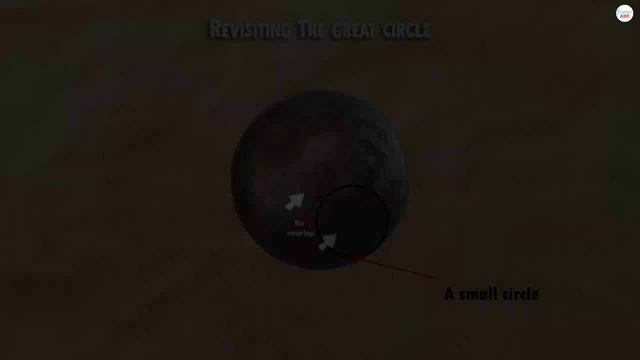 a great circle is the largest circle that can be carved out of a sphere. A small circle, on the other hand, is when the centers of the circle and the sphere do not coincide side. Imagine cutting the Earth along the equator or the poles, The resulting hemispheres.